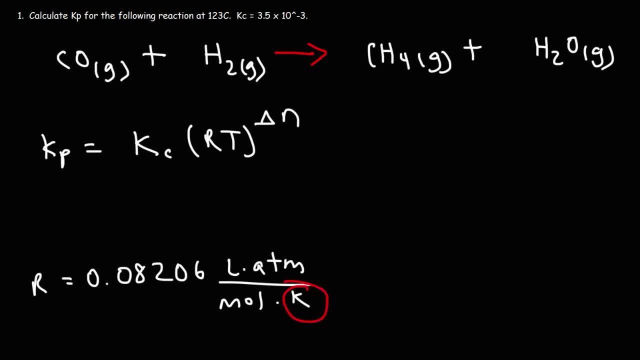 Now note that the unit of temperature is in Kelvin. Right now we have the temperature in Celsius, so we need to convert it to Kelvin. The Kelvin temperature is equal to the Celsius temperature plus 273.. So we need to add 123 and 273, and that is going to be 396 Kelvin. 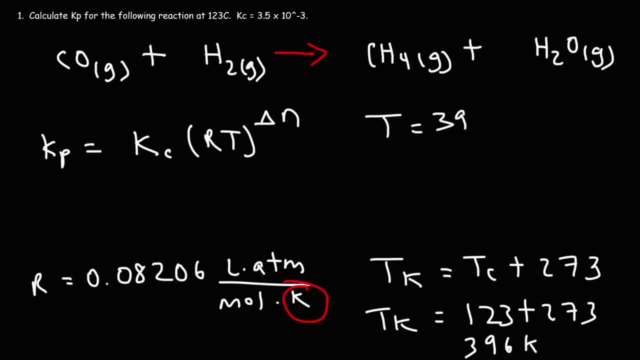 So that's our T value in this problem. Now you might be wondering: what about delta N? What is delta N? Delta N is the difference between the sum of the coefficients of the products minus the sum of the coefficients of the reactants. 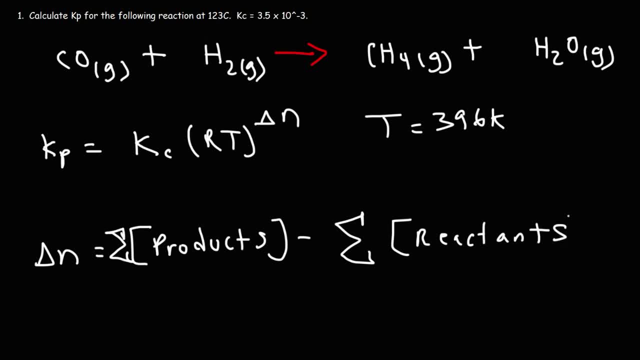 So in order to calculate delta N, we need to balance the chemical equation first. Now, when balancing a chemical equation, it's best to save the substance in its pure elemental form. Las. Notice that hydrogen is in its pure elemental form, So I would balance that element, Las. 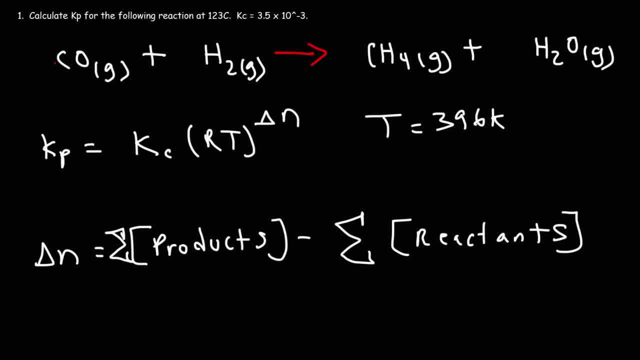 Note that the number of carbon atoms is the same on both sides, So let's put a 1 in front of carbon monoxide and in front of methane. Now notice that we have the same number of oxygen atoms on both sides- It's one, So let's put a one in front of H2O. 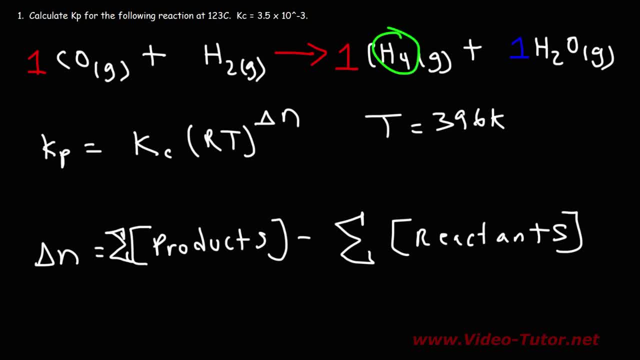 Now notice that we have four hydrogen atoms in methane and two in steam, So that's six on the right side. In order to have six hydrogen atoms on the left side, six divided by two is three, So we need to put a three in front of H2.. So that is the balanced chemical equation. 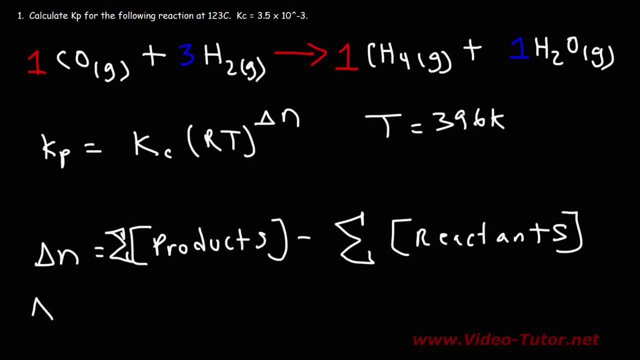 for this reaction. Now the sum of the coefficients of the products. it's going to be one plus one. The sum of the coefficients of the reactants is one plus three, And everything is in its gaseous state, so we can use all of it. 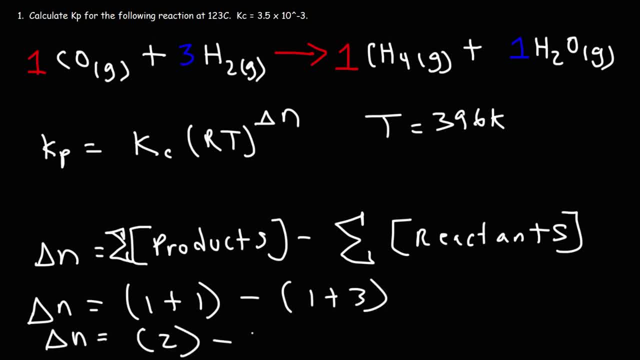 One plus one is two. One plus three is four. So this is one plus three And this is one plus three. This is two minus four, which is equal to negative two. So that's our n value. n is negative two in this example problem. 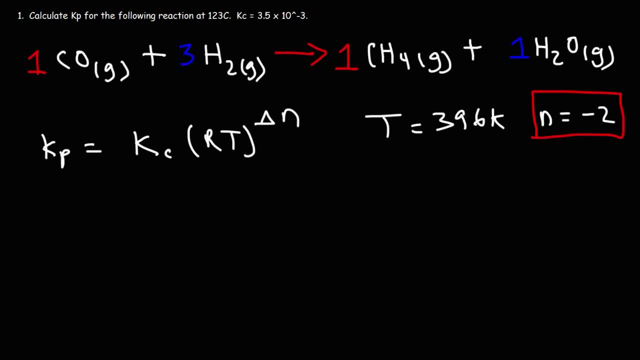 So now that we have that, let's go ahead and plug everything in to this equation. So the equilibrium constant for concentration is 3.5 times 10. to the minus three, Our r value is 0.08206.. And we have a Kelvin temperature of 396.. 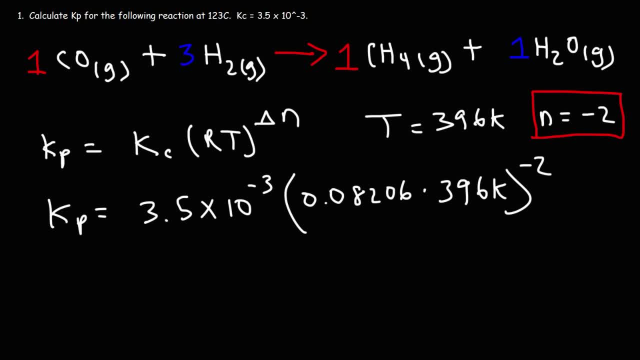 And then delta n. that's negative two. So let's take this one step at a time: 0.08206 times 396.. That's 32.496.. And we're going to raise that to negative two. So once you raise it to the negative, second power: 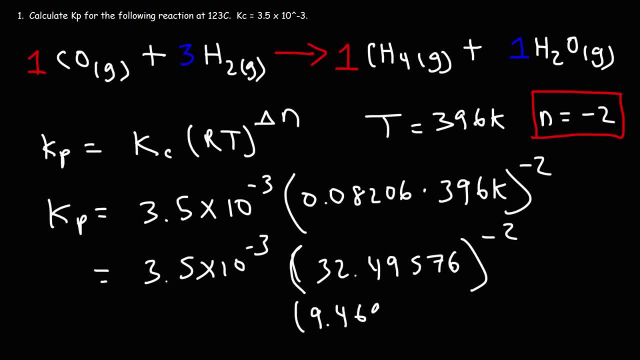 you should get 9.4699 and some other numbers times 10 to the minus four. So if we take that number, multiply it by 3.5, times 10 to the minus three, This gives us the equilibrium constant for partial pressure. 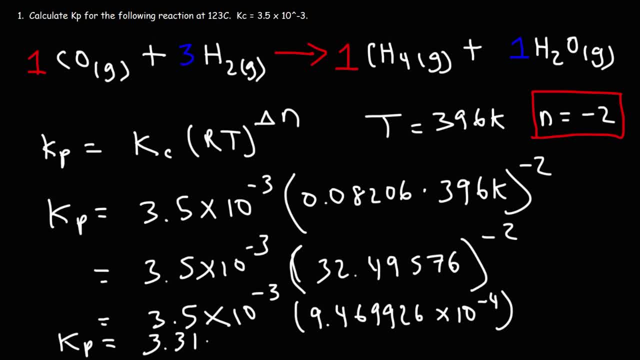 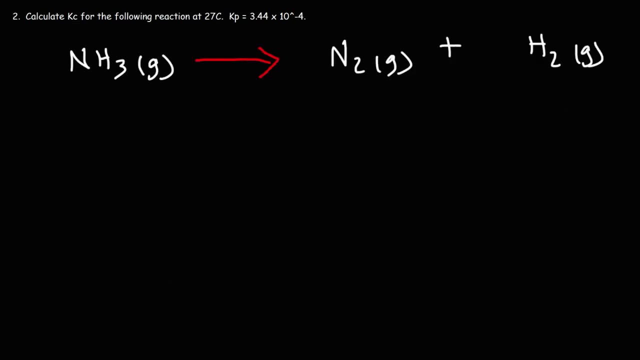 which is 3.314 times 10 to the minus six. So this is our Kp value. So now you know how to calculate Kp given Kc. Here's another example: Kc, the equilibrium constant for concentration, given Kp. 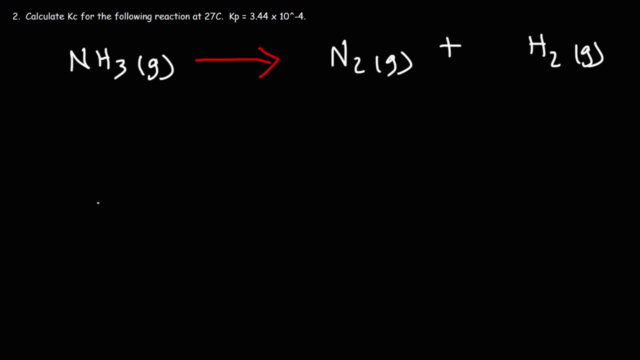 Feel free to pause the video if you want to try it. So, going back to our original formula, we know that Kp is equal to Kc times RT raised to the delta n. Well, in this example, we want to calculate Kc. 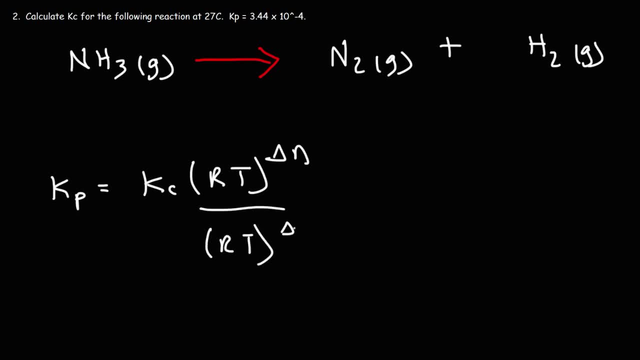 So we need to rearrange this equation. If we divide both sides by, by RT raised to the delta n, we can get the formula for Kc. And so here it is: Kc is equal to Kp divided by RT raised to the delta n. 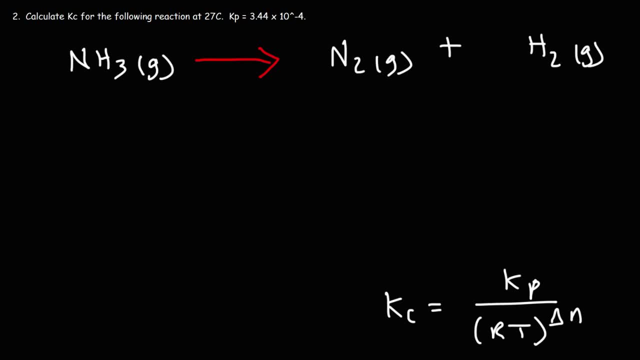